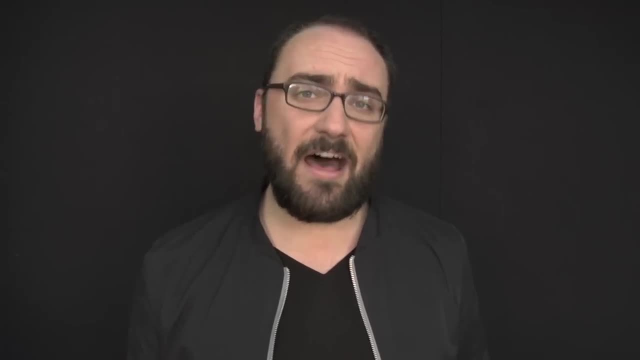 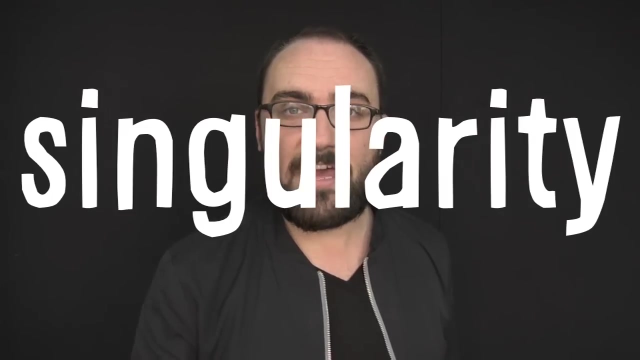 And when it runs out of fuel and can no longer keep itself hot enough, it collapses to a single, infinitesimally small point, known as a singularity. Its density will be infinite, and so its gravitational pull will be so strong that nothing can escape. 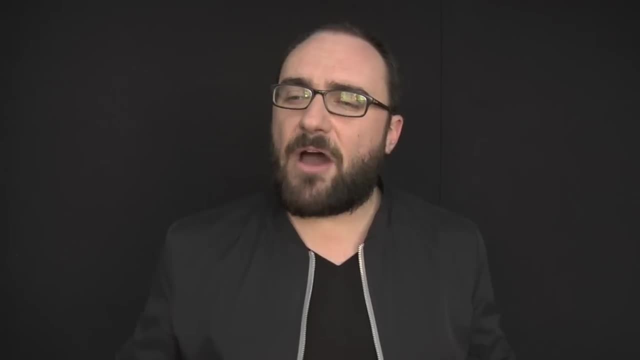 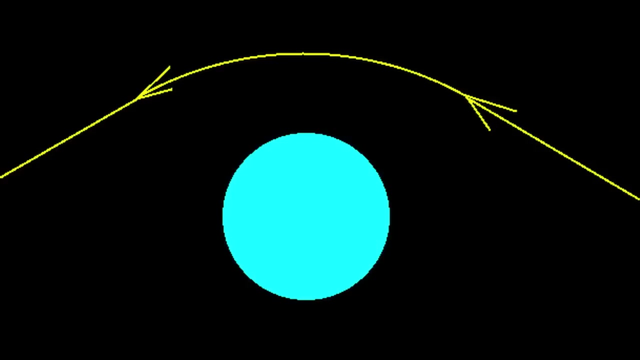 Not even light. But enough about ways black holes form. Let's jump into one First question: what would it look like from the outside? Well, we know that gravitational fields bend space and time. Stars behind our sun will actually appear to be in slightly different locations from Earth. 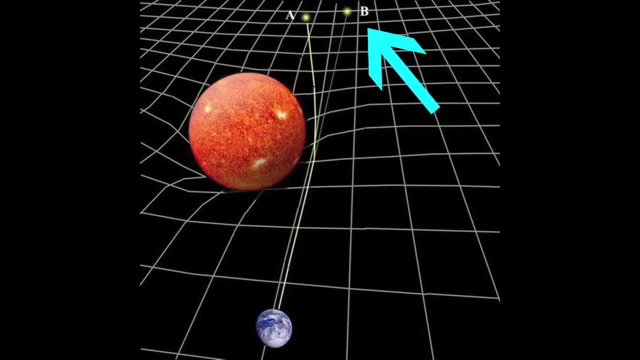 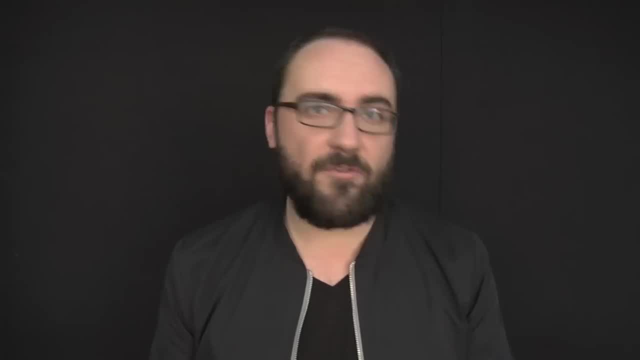 because the sun's gravitational field bends the light coming from those stars. When it comes to the gravitational fields of larger objects like entire galaxies or, for that matter, a black hole, the effect is even nuttier. Light coming from objects behind them is significantly distorted, producing smears and smudges. 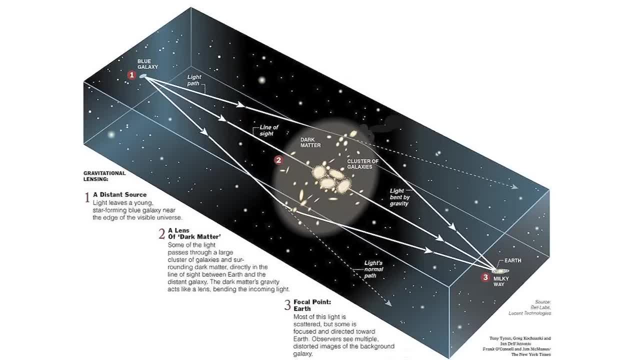 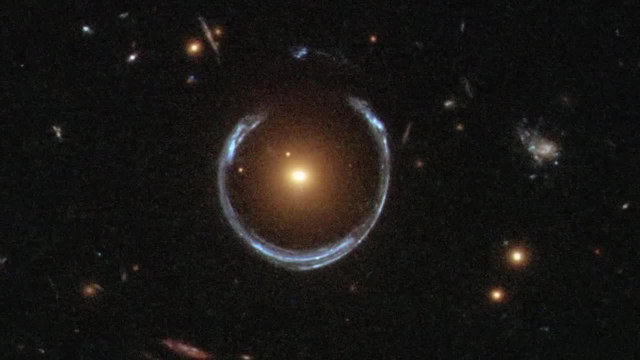 As seen from Earth. the blue galaxy behind this red galaxy is completely distorted, like a funhouse mirror. So, rather than appearing as it really should, it looks to us like a ring, a smudge all the way around the red galaxy. This is known as gravitational force. 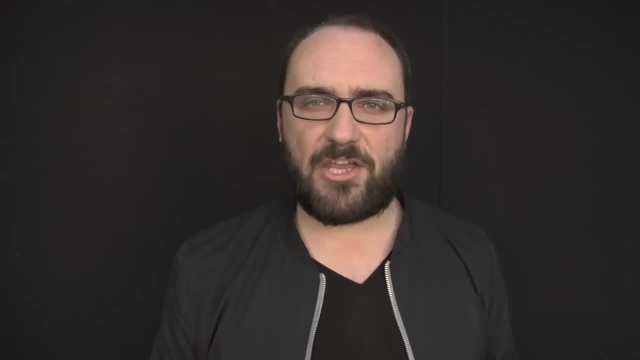 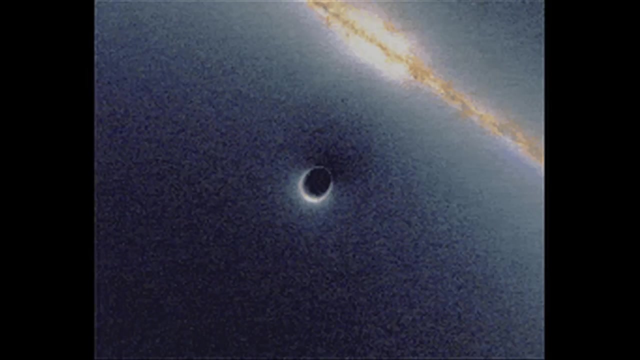 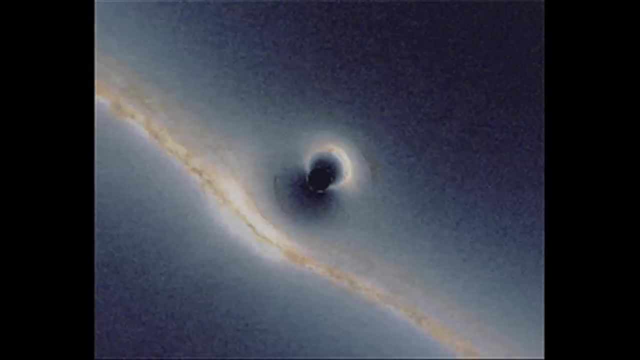 Or gravitational lensing. Now take a look at this simulation of a black hole with a galaxy millions of light years behind it. The galaxy's not really in danger of the black holes suck, but the light coming off of that galaxy certainly is. Watch as the galaxy passes behind the black hole. 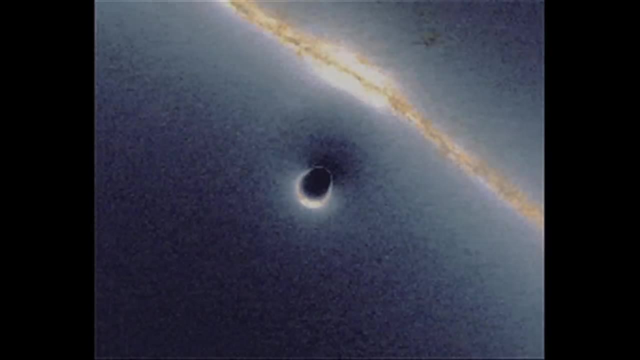 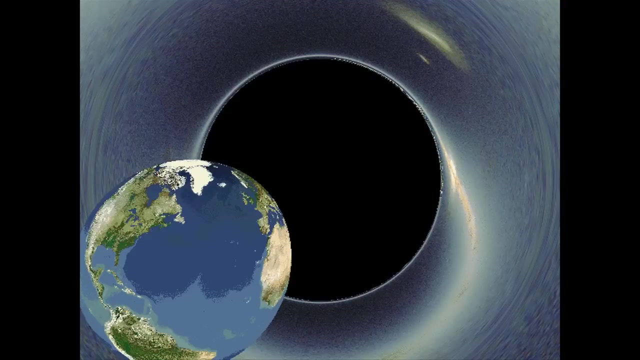 and its light is contorted, twisted and distorted. Now here's a really fun demonstration. What if the Earth were to orbit around a black hole? Looking from the outside, the Earth would look normal at first, but as soon as it passed behind the black hole, 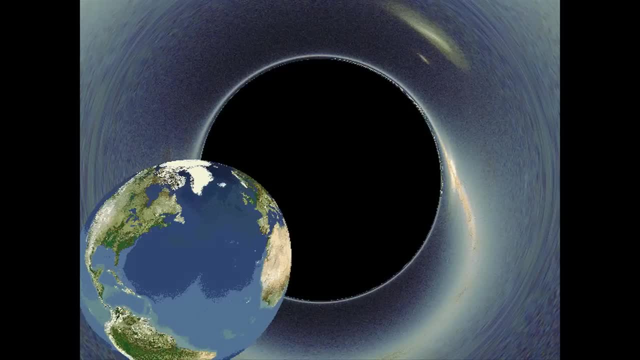 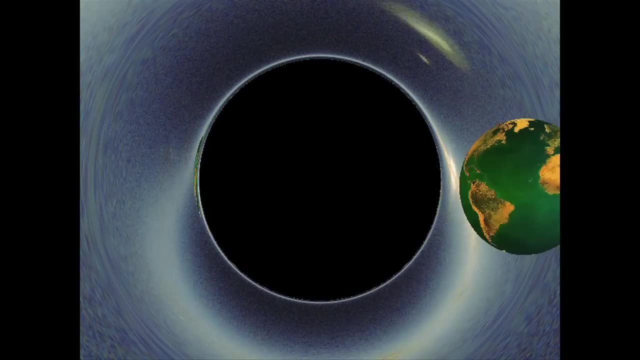 the black hole's gravitational field would warp the light reflecting off the Earth, producing this. For the sake of simplicity, let's jump into a simple black hole, One that doesn't have a charge and isn't moving And also isn't already sucking up a bunch of matter. 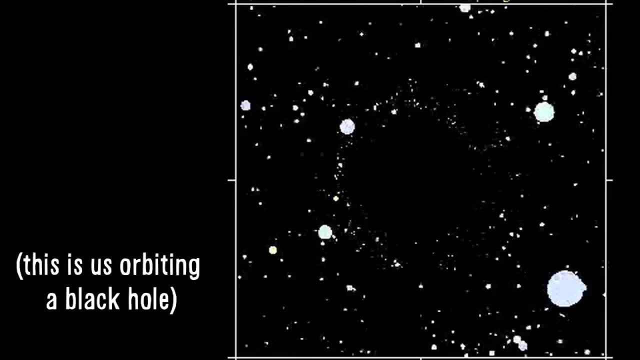 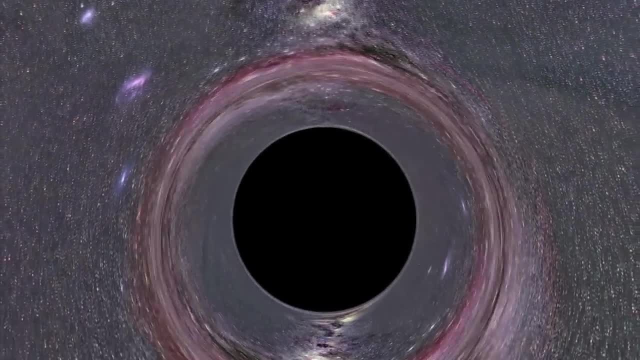 So it's just there on its own. As we approach, the distortion of the sky grows greater and greater. A larger and larger portion of our galaxy, a larger and larger portion of our field of view looking forward into the black hole, will be filled with darkness. 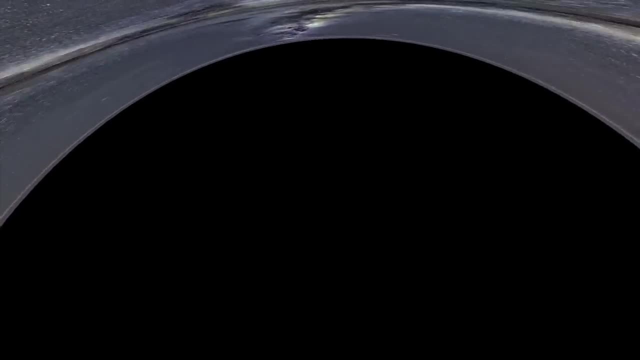 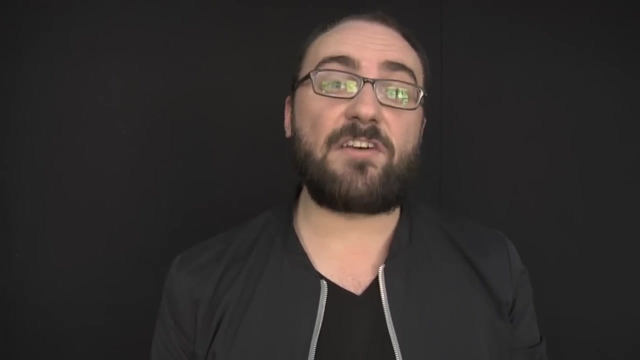 At this point, where half of our field of view has been swallowed up in darkness, we have reached the photon sphere. At this point, light is not going to necessarily get sucked into the black hole, but it doesn't necessarily leave it either. 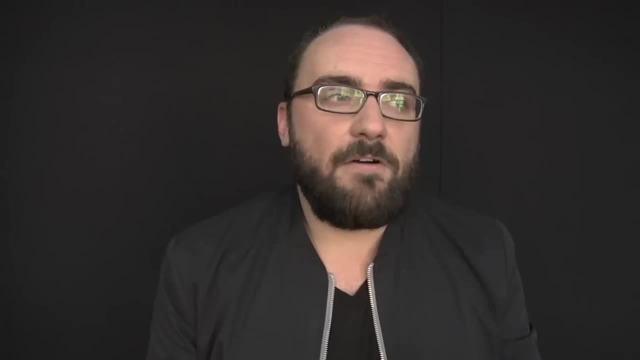 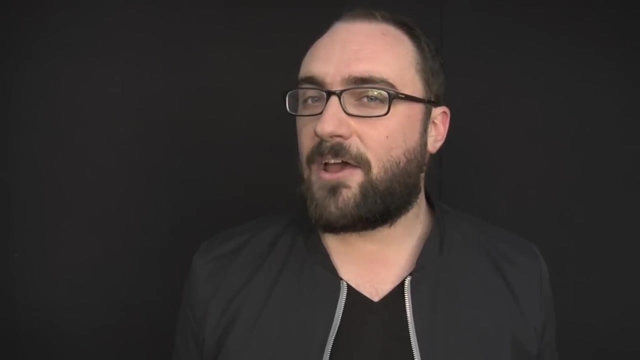 Instead, at this magical point in space, light photons can actually orbit the black hole. If you were to stop here for a moment and look to the side, you could theoretically see the back of your own head, Because light reflecting off the back of your head. 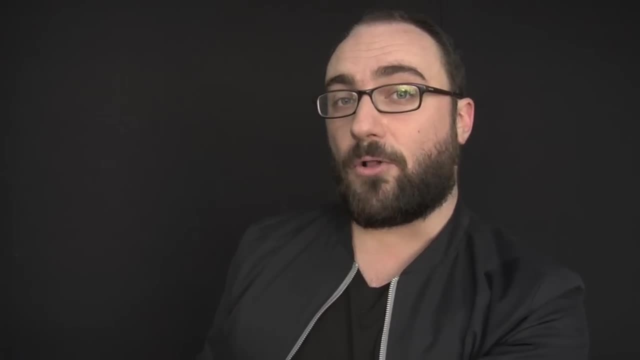 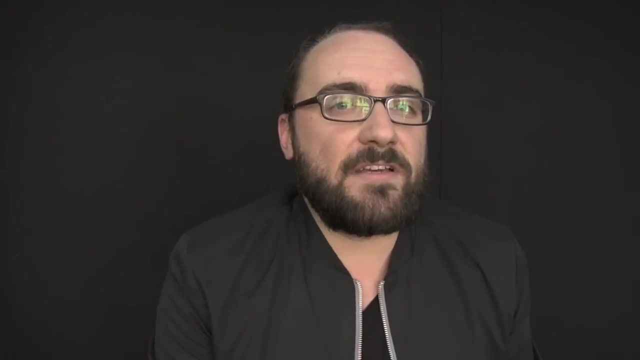 would travel all the way around the sphere of the black hole right back to your face. A gravitational field not only warps space, it also warps time. Now, for most intents and purposes, here on Earth, we never have to worry about that. 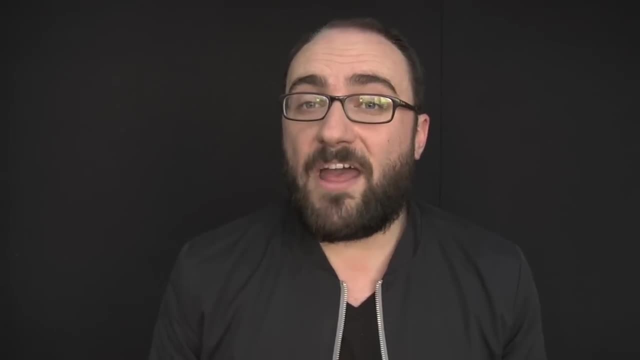 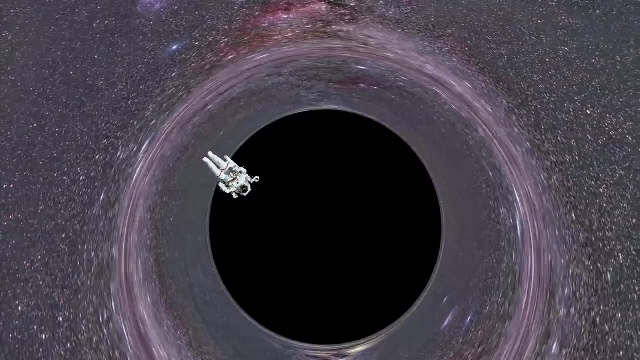 But near a black hole, gravity would be so strong that an observer standing watching you jump into the hole would see something quite strange. They wouldn't see you get sucked quickly into the hole. Instead, they would see your approach become slower and slower and slower. 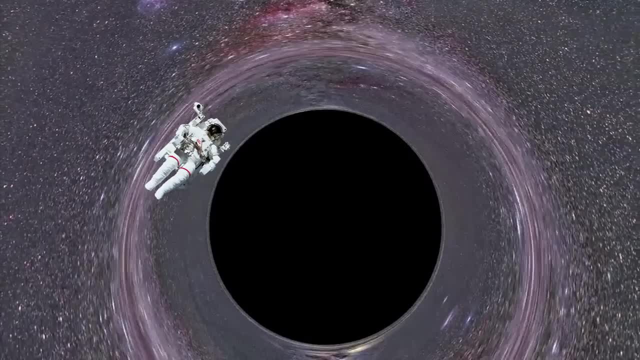 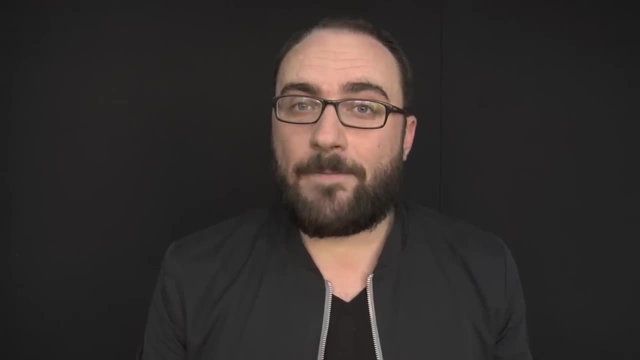 until you reached a point known as the event horizon. This is a point in space where, once crossed, there's no going back. It is at that point that light can no longer escape, And so to a person watching you fall into the hole, 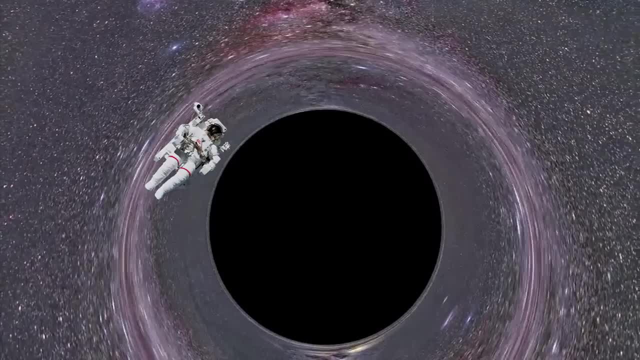 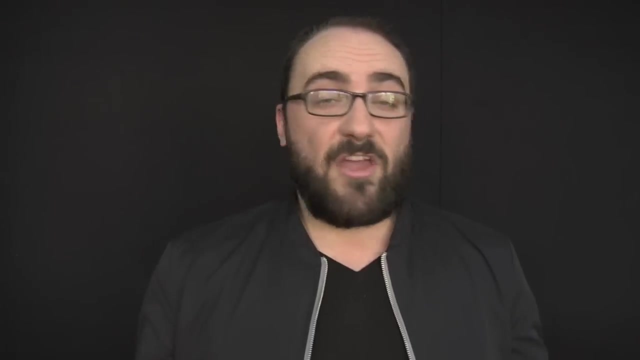 that would be where your journey ended. You would seem almost frozen in space, the light coming off your body becoming increasingly red-shifted until you simply faded into nothingness. They would never see you cross the event horizon, But for you, of course, everything would seem fine and dandy. 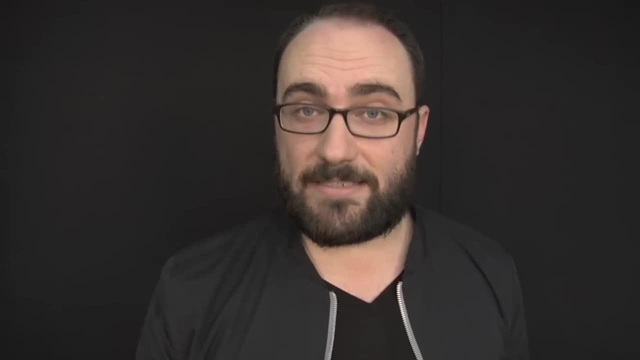 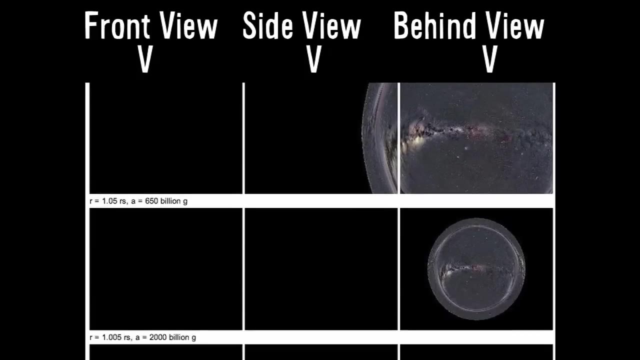 You would continue past that horizon to your now inevitable death. As you continue to approach the black hole's singularity, your view of the entire universe would get compressed into a smaller and smaller point in space behind you, If the black hole we're jumping into. 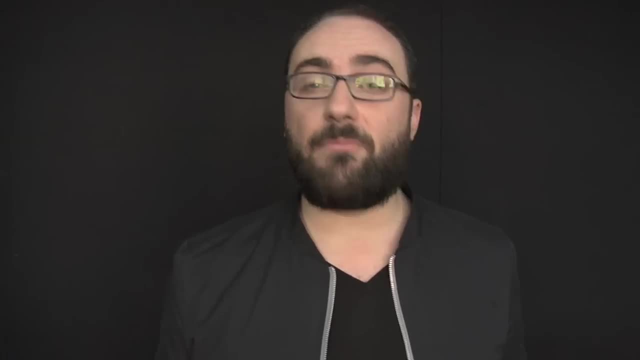 is large enough, things might actually be quite comfortable. at that event horizon We'll know that we're never going to escape and that our lives are pretty much over. but it might take us hours to actually reach a point where things started to hurt. 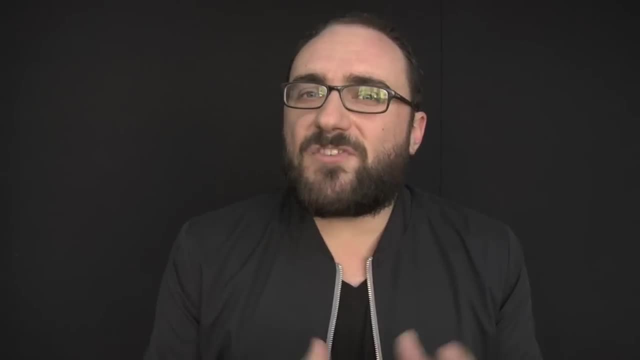 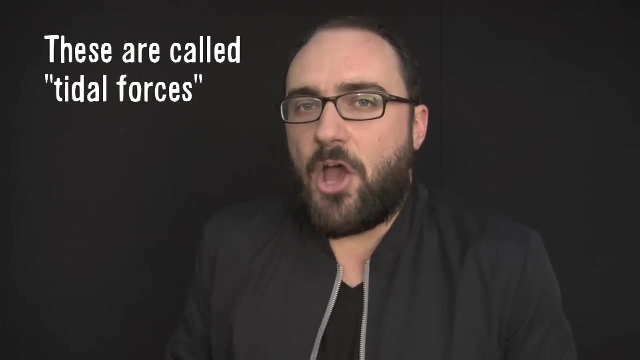 Why would they hurt? Well, the closer you get to the singularity, the more significant the difference in gravitational pull is across space, And so parts of me that are closer to the singularity would be pulled more strongly than parts that were facing away. 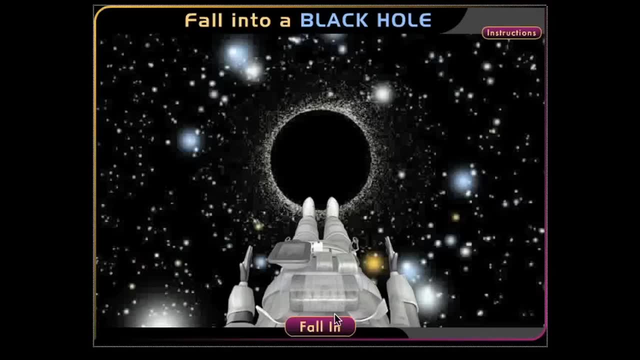 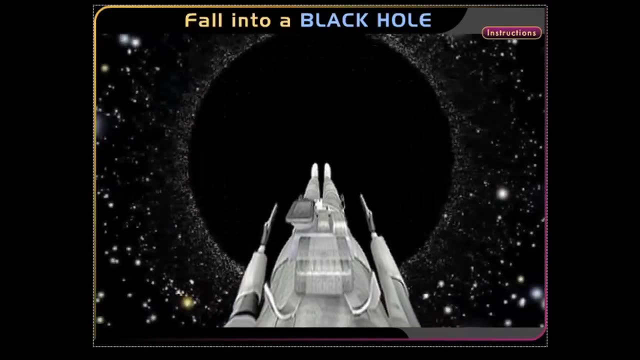 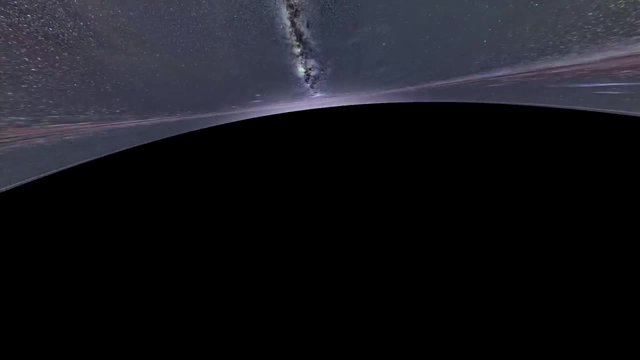 and my entire body would be stronger, would be stretched toward the singularity. The effect would be so incredible. scientists don't usually call it stretching, they call it spaghettification. Once you reach this point, you would be dead. Your molecules would be violently ripped and stretched apart. 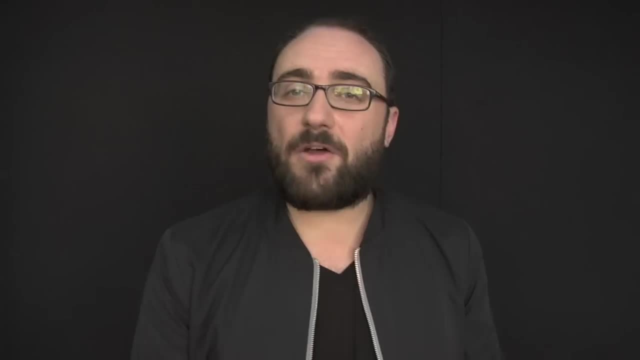 and when they got to the singularity? well, we don't really know what would happen. Perhaps they would completely disappear, in violation of all the laws of physics, or maybe they would reappear elsewhere in the universe. It's believed that a moving or spinning black hole 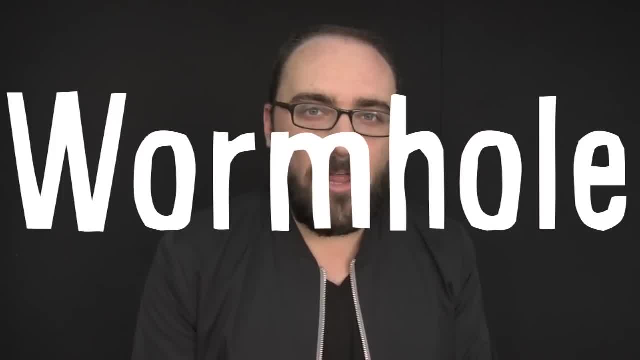 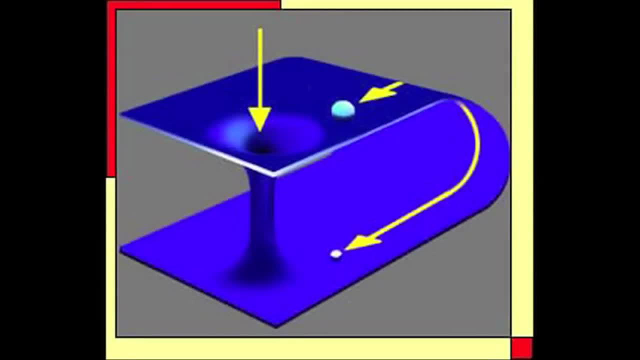 might actually create what is known as a wormhole, a way of transitioning across space faster than light, Not in any way that violates the laws of science, but in a way that takes advantage of the universe's dimensions, For instance. if I wanted to get from this point to this point, I'd have to travel the distance. But theoretically a wormhole would do something really crazy, For instance this: Now the two parts of me are right next to each other and I can travel between them almost instantaneously, But again, this is all theoretical. 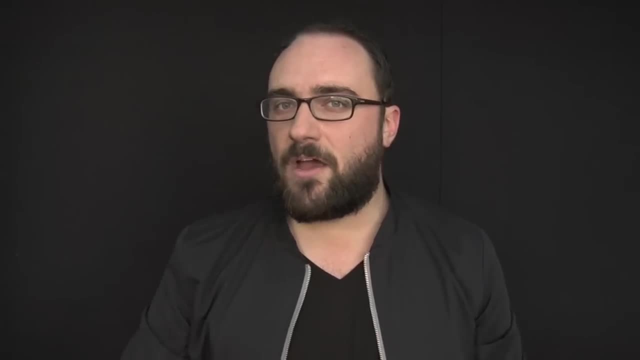 Luckily, we do have a possible way of analyzing black holes right here on Earth. Enter the dumbhole. Just as a black hole does not permit light to escape, a dumbhole is an acoustic black hole. It won't allow sound to escape. 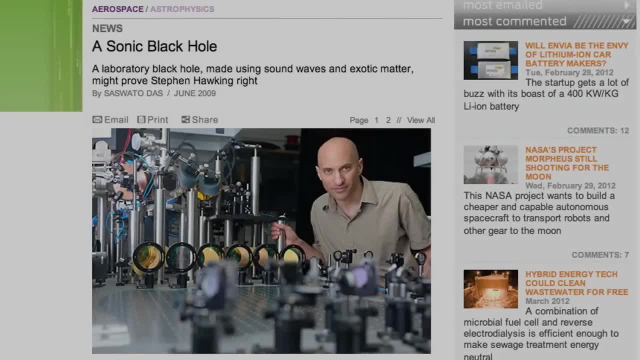 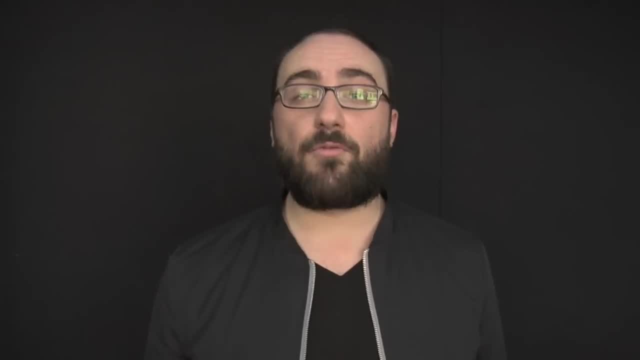 It doesn't have to be nearly as powerful, and scientists have been able to create dumbholes in laboratories using special fluids traveling at the speed of sound. A lot of progress still needs to be made in the world of acoustic black holes, but we may be able to learn an amazing amount of information. 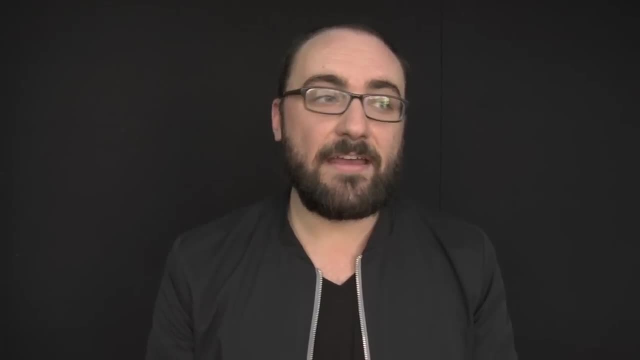 about how black holes work by looking at how sound is treated in a dumbhole. Now here's another good question: What would it look like to travel at the speed of light, say, toward the sun? Well, surprisingly, you wouldn't just see the sun. immediately rush up toward you. No, no, no. In fact, initially it would look almost as if the sun were receding away from you. Why? Because your field of view would vastly increase in size. You would be able to see stuff almost behind you. And here's why, As you sit there, not moving yet looking at the sun, there's light coming from stuff behind you. But if you travel the speed of light, you will actually reach that light coming from things behind you As you reach light speed. 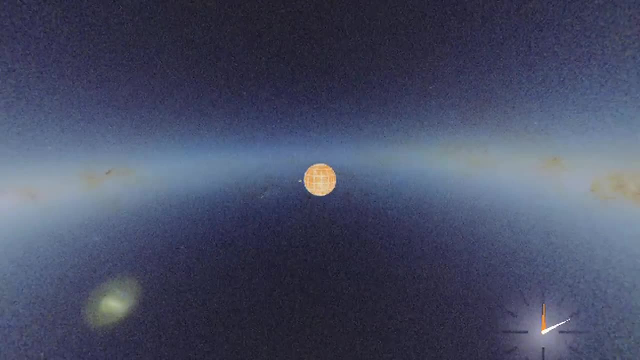 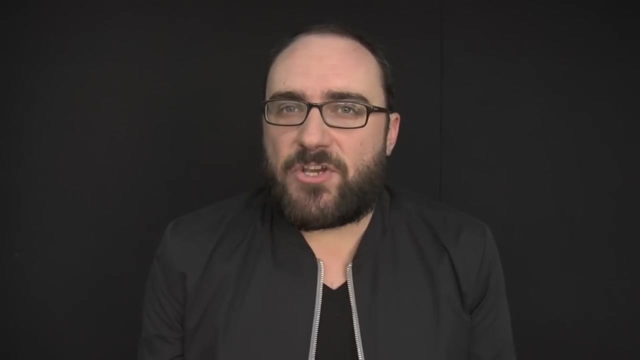 your field of view would expand like this, concentrating the stuff in the middle. But where are you in the universe? Or here's a better question: Where is the center of the universe? Well, this might sound crazy, but it's everywhere. 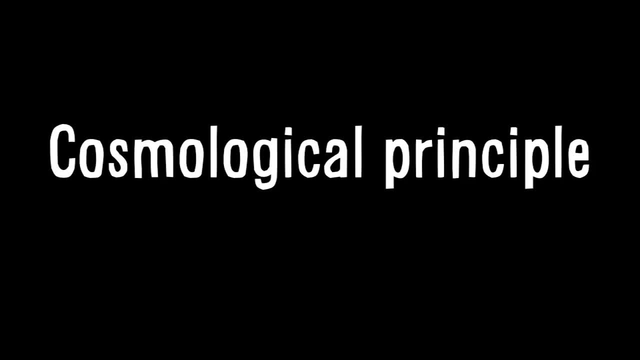 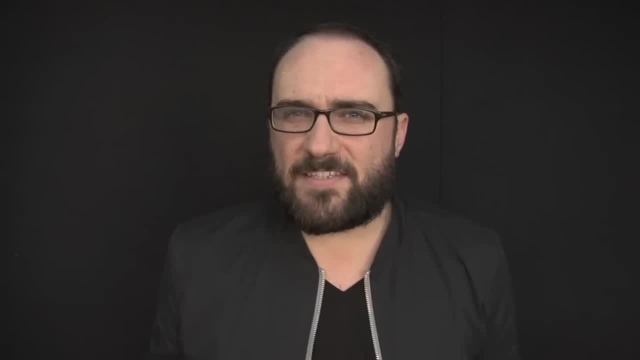 This is known as the cosmological principle: No matter where you are in the universe, everything else will seem to be moving away from you, expanding at the same rate. The universe is expanding, but not like a balloon getting bigger with all the people inside it. 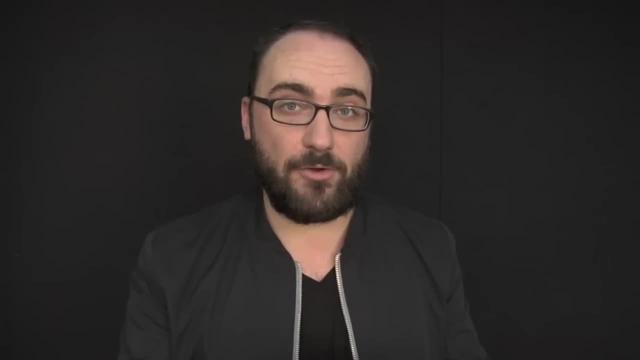 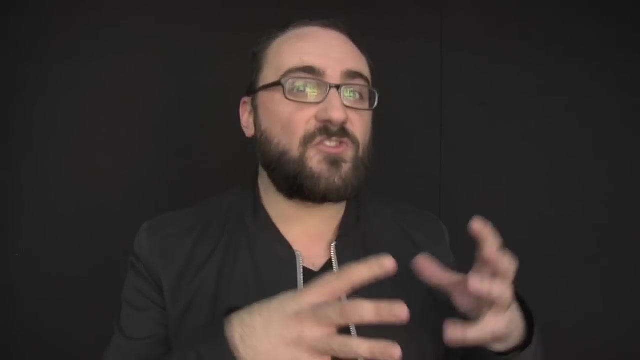 Instead, it's as if we are the surface of a balloon. If you were to put a bunch of dots on a balloon and then blow it up, all of the dots would move away from each other at the same rate. And on the surface of the balloon. 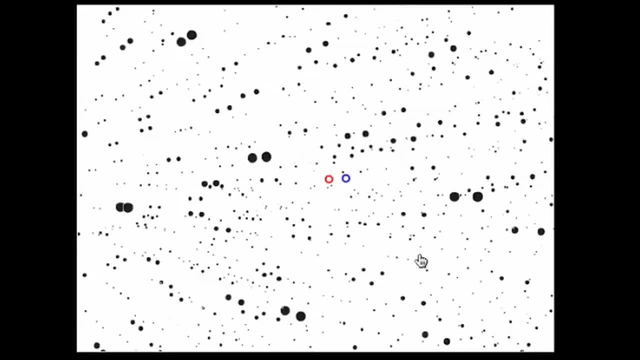 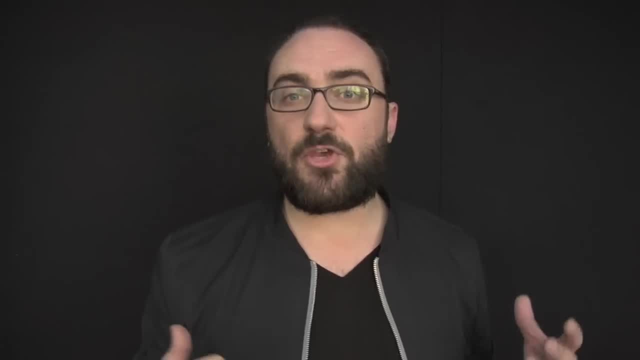 there is no center. Take a look at these two layers. They are exactly similar, except the top layer represents a 5% expansion of the bottom layer. Let's say that you live on one of these dots and you want to measure where everything's moving away from. 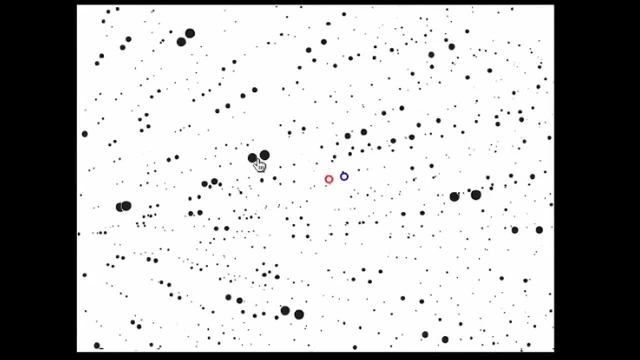 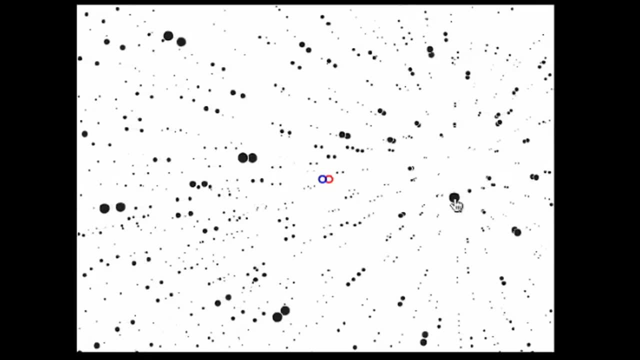 Well, watch what happens when I line up a dot in the past and the present Boom. It looks like the center of the expansion. I can do this with any dot, As soon as I choose a dot to be the frame of reference. 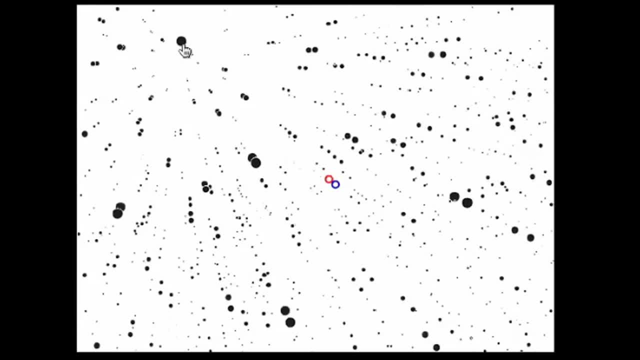 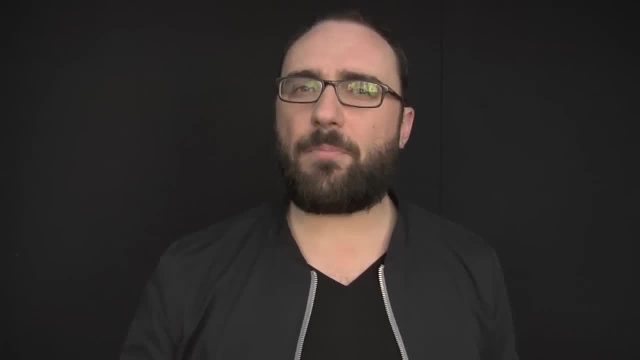 it immediately becomes the center of the expansion. So, while dying in a black hole would be lonely and scary and morbid, when you look up into the sky, think instead about this, No matter where you are or who you are, or what your friends or your parents tell you. 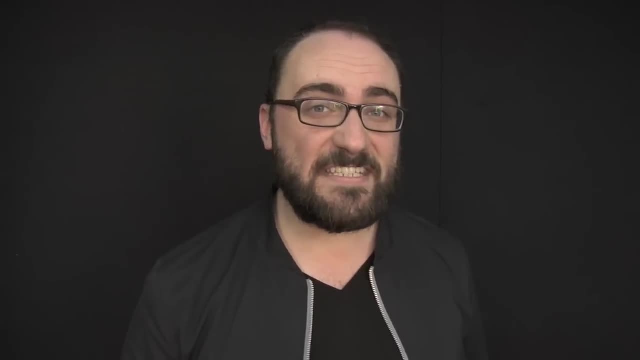 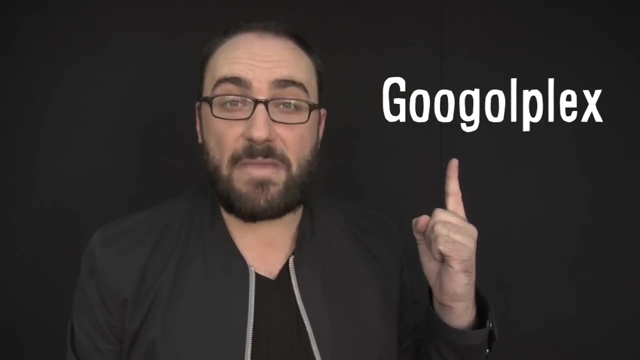 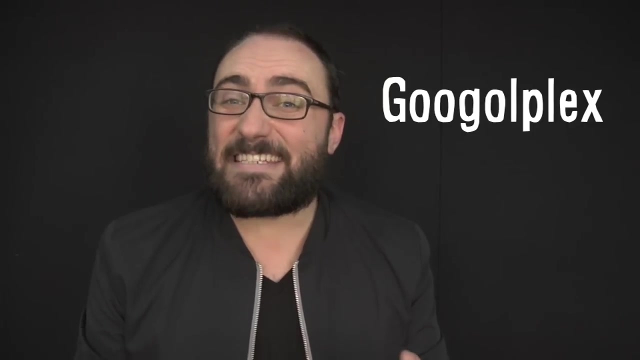 you really, scientifically, are the center of the universe. Finally, what if our universe was a googolplex meters across? It is nowhere near that large, But if it was, it would be so voluminous that statistically it would be nearly impossible. 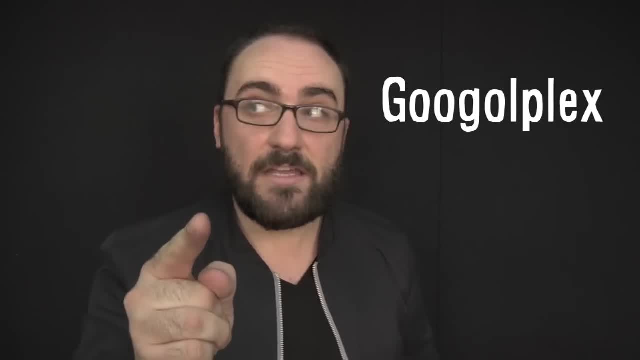 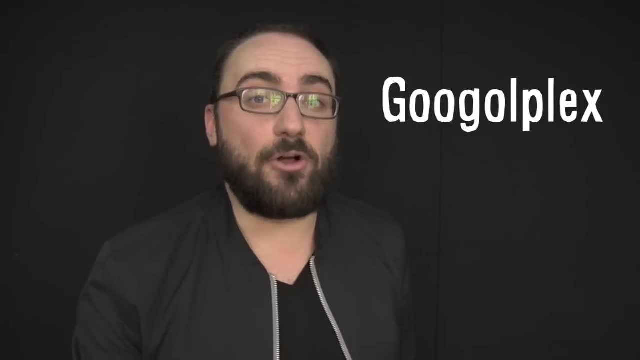 for there not to be an exact copy of you somewhere else out there in the universe. To see why, I highly suggest that you click right there and check out Brady Heron's new channel, Numberphile. It's part of the YouTube Original Channels.